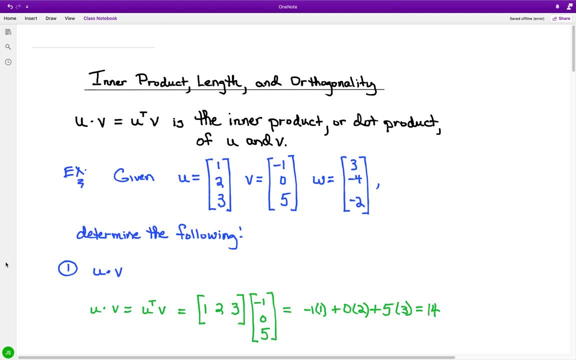 Okay, we have what will be referred to as inner product length and orthogonality, And much of this stuff is going to be carried over from what we have had at the end of Math 172, where we had dealing with vectors, dot products and so on. 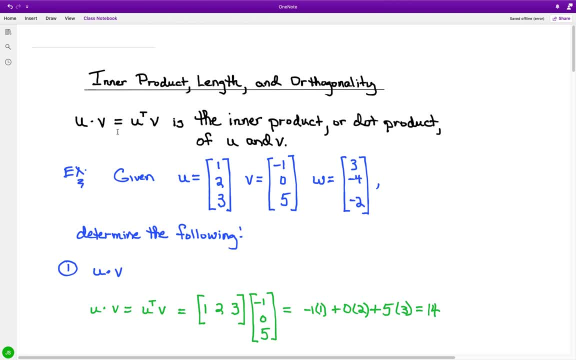 Okay, we have what will be referred to as inner product length and orthogonality, And much of this stuff is going to be carried over from what we have had at the end of Math 172, where we had dealing with vectors, dot products and so on. 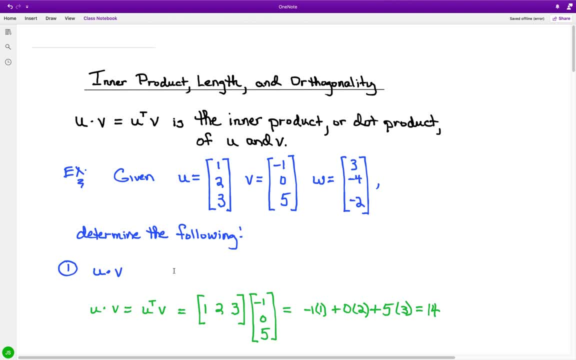 Okay, we have what will be referred to as inner product length and orthogonality, And much of this stuff is going to be carried over from what we have had at the end of Math 172, where we had dealing with vectors, dot products and so on. 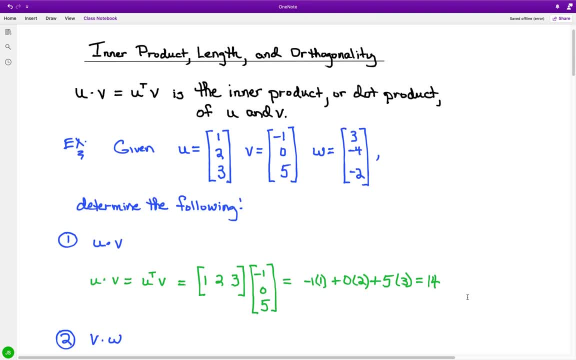 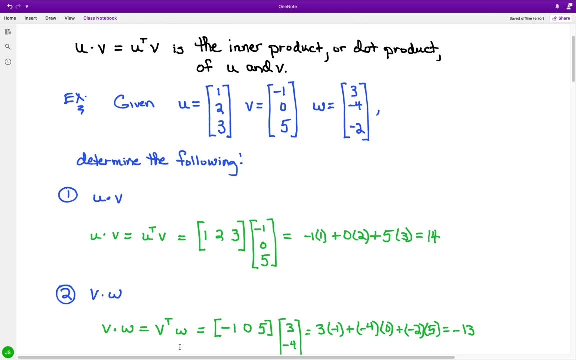 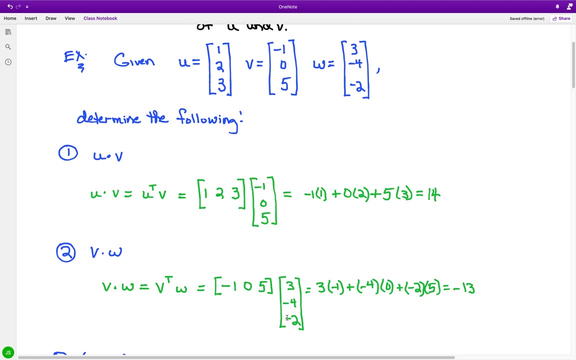 Okay, we have what will be referred to as inner product length and orthogonality, And much of this stuff is going to be carried over from what we have had at the end of Math 172, where we had dealing with vectors, dot products and so on. 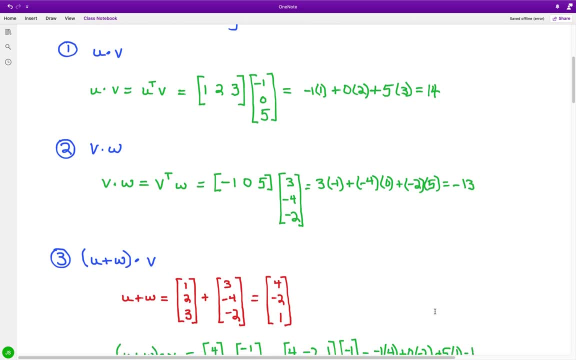 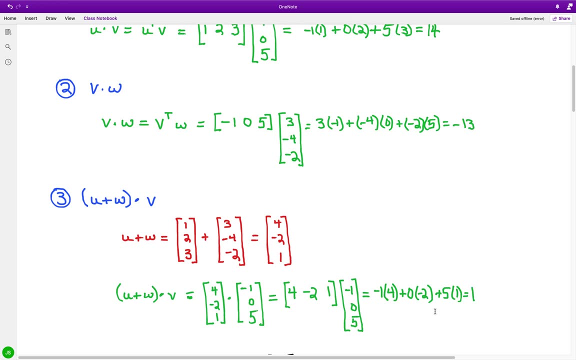 Okay, we have what will be referred to as inner product length and orthogonality, And much of this stuff is going to be carried over from what we have had at the end of Math 172, where we had dealing with vectors, dot products and so on. 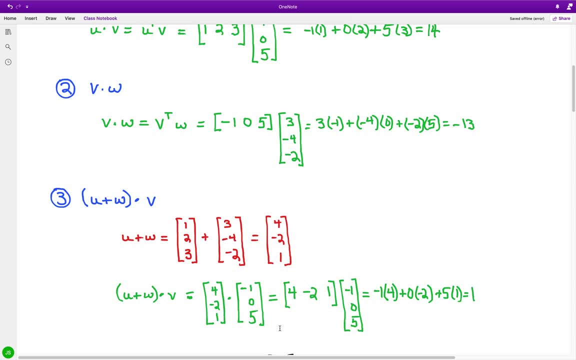 Okay, we have what will be referred to as inner product length and orthogonality, And much of this stuff is going to be carried over from what we have had at the end of Math 172, where we had dealing with vectors, dot products and so on. 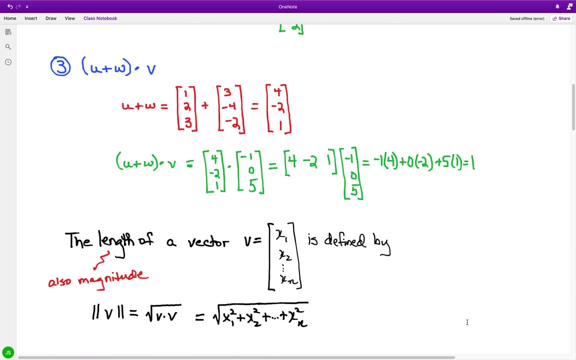 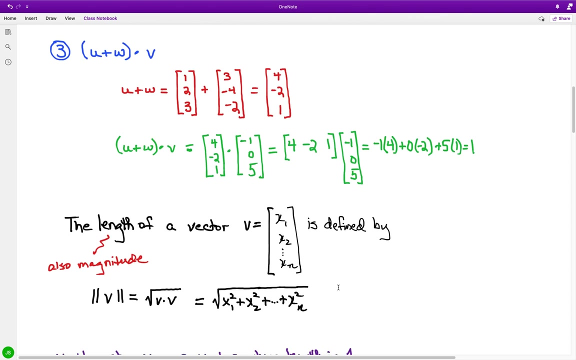 Okay, we have what will be referred to as inner product length and orthogonality, And much of this stuff is going to be carried over from what we have had at the end of Math 172, where we had dealing with vectors, dot products and so on. 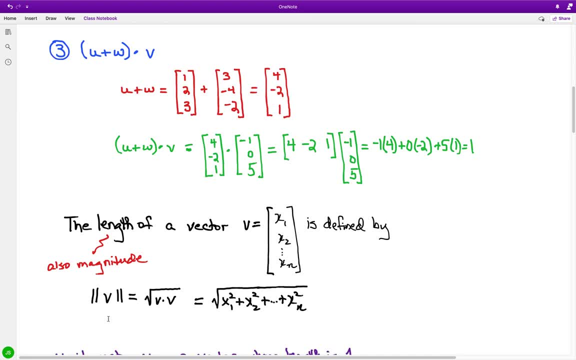 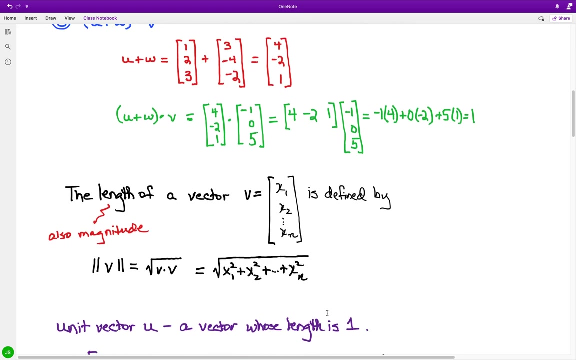 Okay, we have what will be referred to as inner product length and orthogonality, And much of this stuff is going to be carried over from what we have had at the end of Math 172, where we had dealing with vectors, dot products and so on. 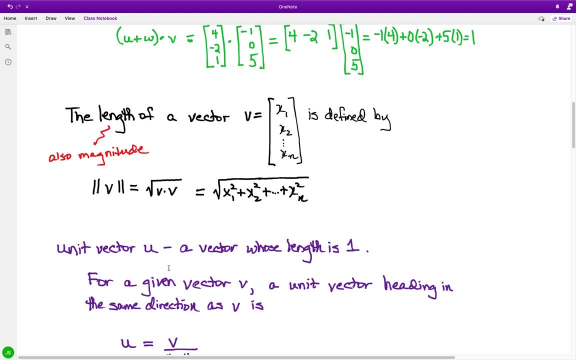 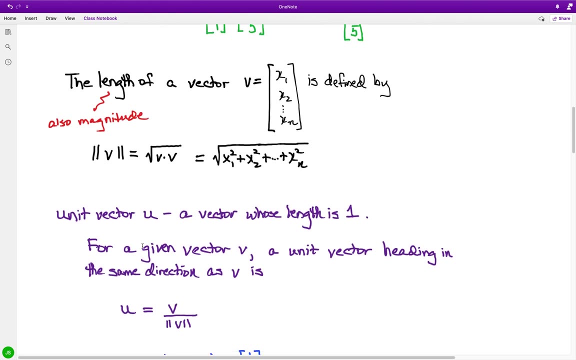 Okay, we have what will be referred to as inner product length and orthogonality, And much of this stuff is going to be carried over from what we have had at the end of Math 172, where we had dealing with vectors, dot products and so on. 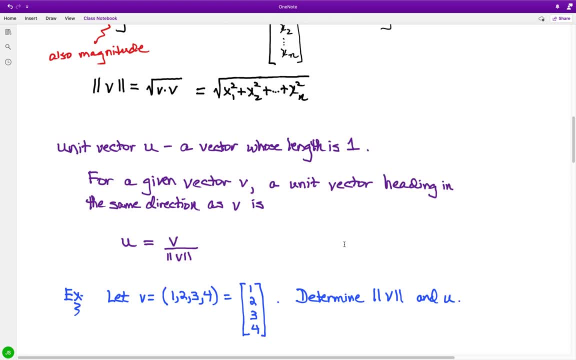 Okay, we have what will be referred to as inner product length and orthogonality, And much of this stuff is going to be carried over from what we have had at the end of Math 172, where we had dealing with vectors, dot products and so on. 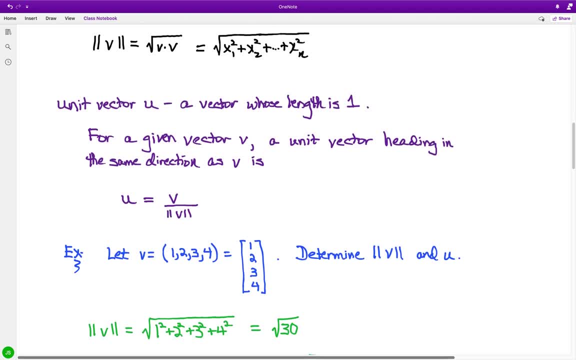 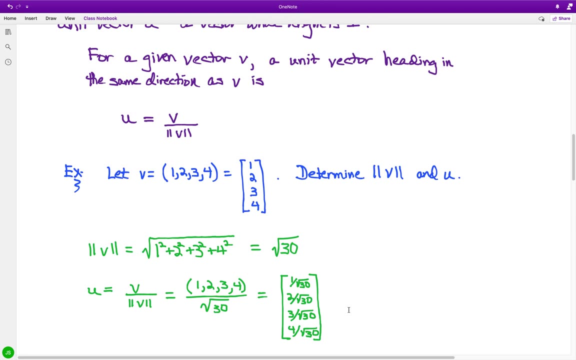 Okay, we have what will be referred to as inner product length and orthogonality, And much of this stuff is going to be carried over from what we have had at the end of Math 172, where we had dealing with vectors, dot products and so on. 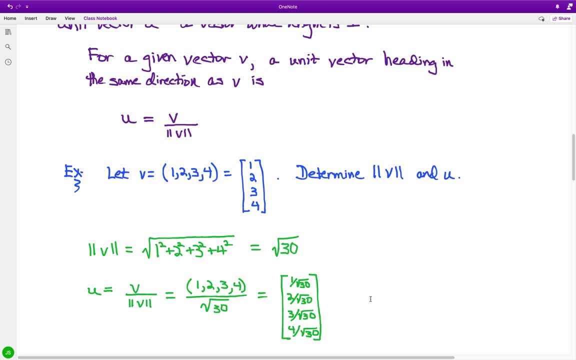 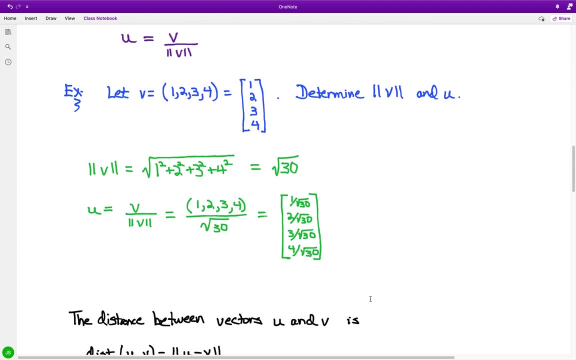 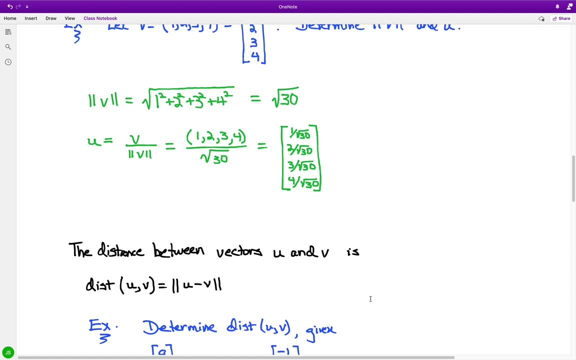 Okay, we have what will be referred to as inner product length and orthogonality, And much of this stuff is going to be carried over from what we have had at the end of Math 172, where we had dealing with vectors, dot products and so on. 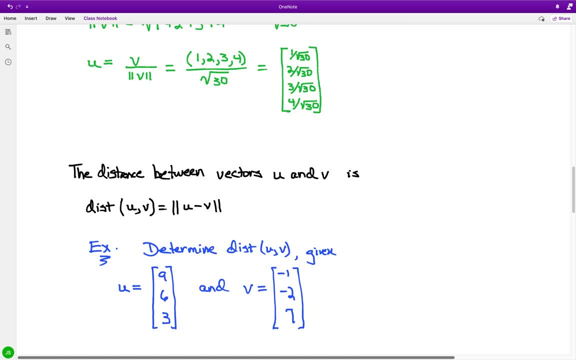 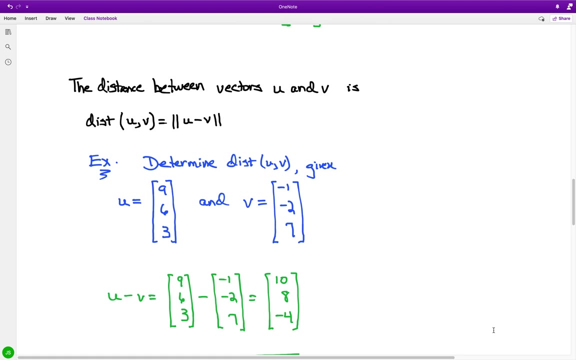 Okay, we have what will be referred to as inner product length and orthogonality, And much of this stuff is going to be carried over from what we have had at the end of Math 172, where we had dealing with vectors, dot products and so on. 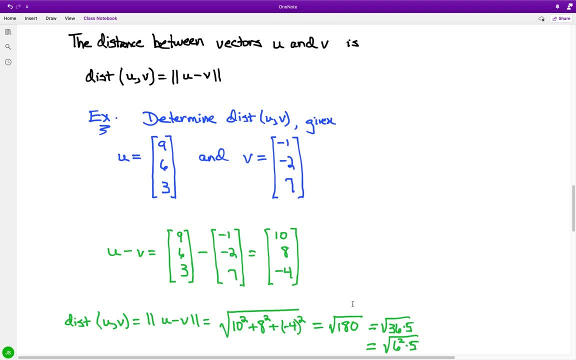 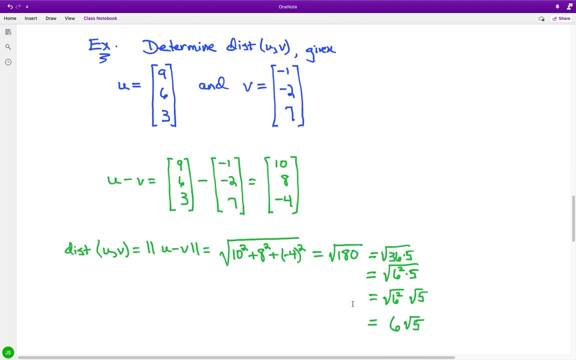 Okay, we have what will be referred to as inner product length and orthogonality, And much of this stuff is going to be carried over from what we have had at the end of Math 172, where we had dealing with vectors, dot products and so on. 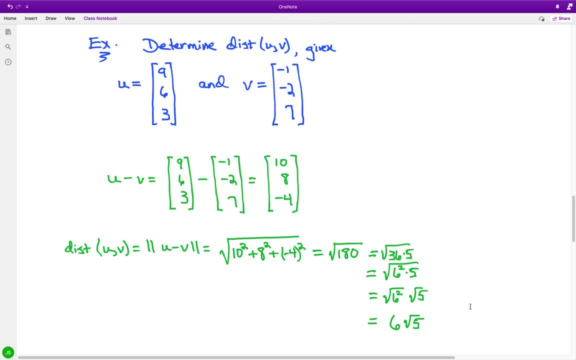 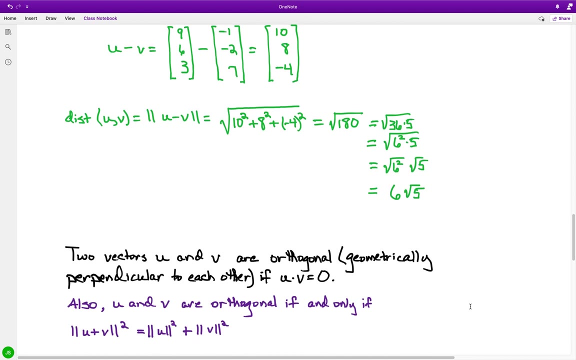 Okay, we have what will be referred to as inner product length and orthogonality, And much of this stuff is going to be carried over from what we have had at the end of Math 172, where we had dealing with vectors, dot products and so on. 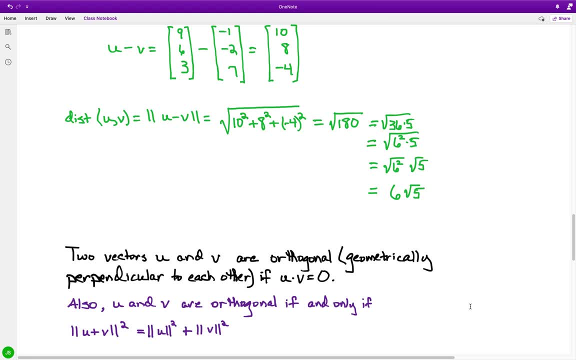 Okay, we have what will be referred to as inner product length and orthogonality, And much of this stuff is going to be carried over from what we have had at the end of Math 172, where we had dealing with vectors, dot products and so on. 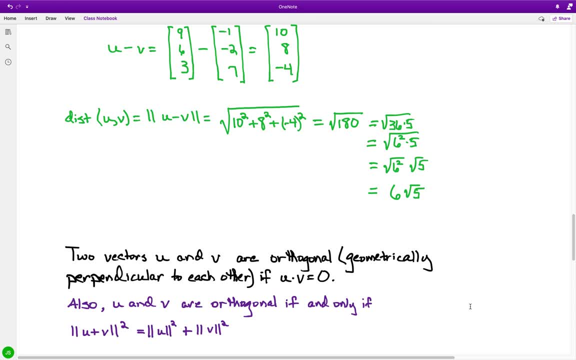 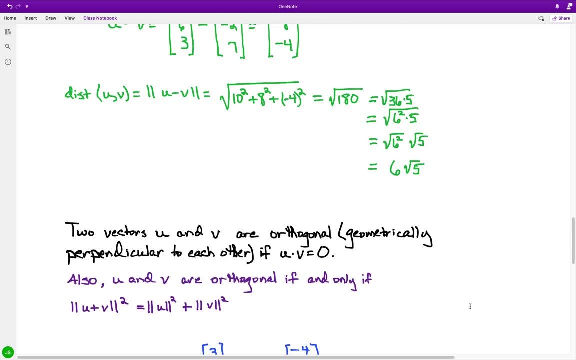 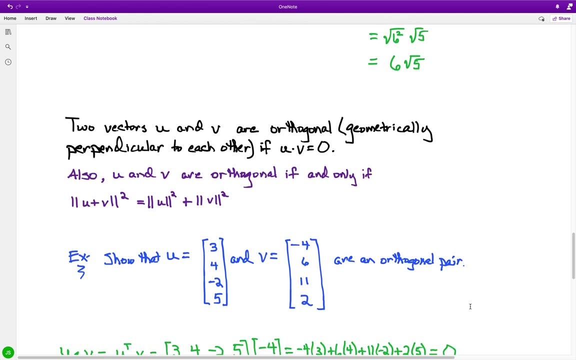 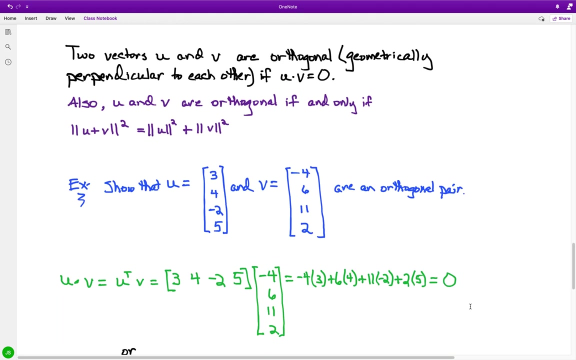 Okay, we have what will be referred to as inner product length and orthogonality, And much of this stuff is going to be carried over from what we have had at the end of Math 172, where we had dealing with vectors, dot products and so on. 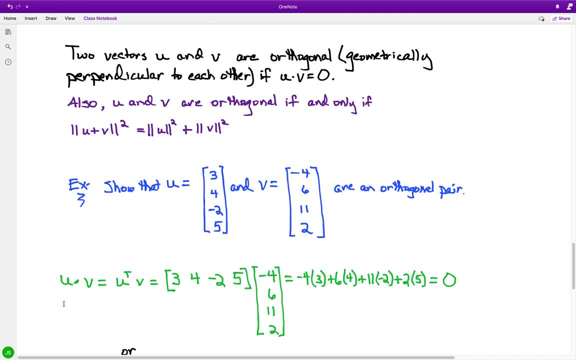 Okay, we have what will be referred to as inner product length and orthogonality, And much of this stuff is going to be carried over from what we have had at the end of Math 172, where we had dealing with vectors, dot products and so on. 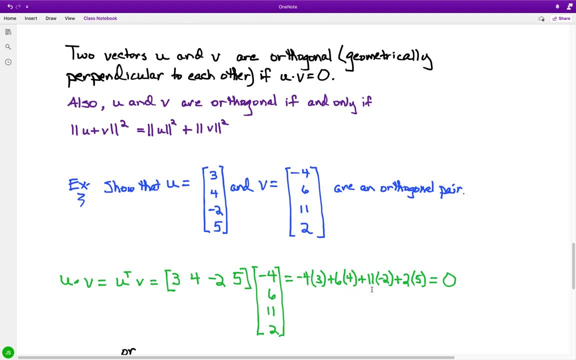 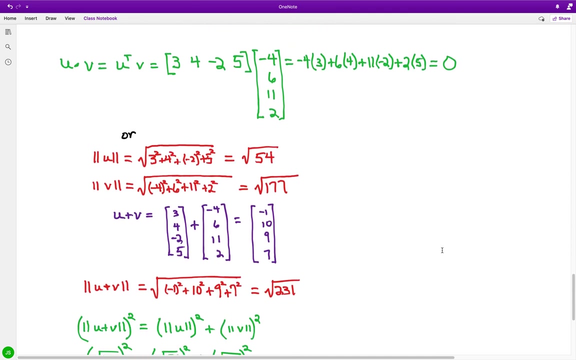 Okay, we have what will be referred to as inner product length and orthogonality, And much of this stuff is going to be carried over from what we have had at the end of Math 172, where we had dealing with vectors, dot products and so on. 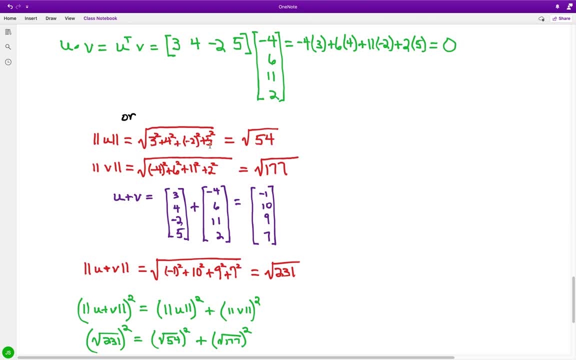 Okay, we have what will be referred to as inner product length and orthogonality, And much of this stuff is going to be carried over from what we have had at the end of Math 172, where we had dealing with vectors, dot products and so on.